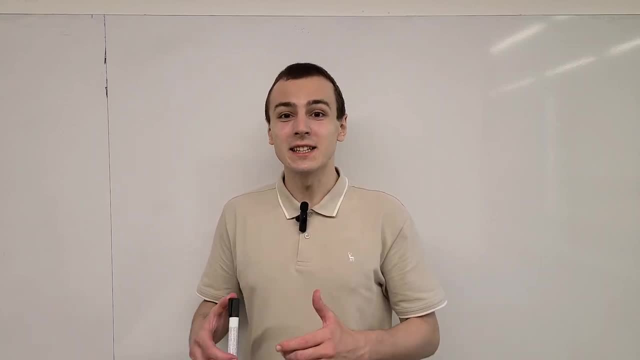 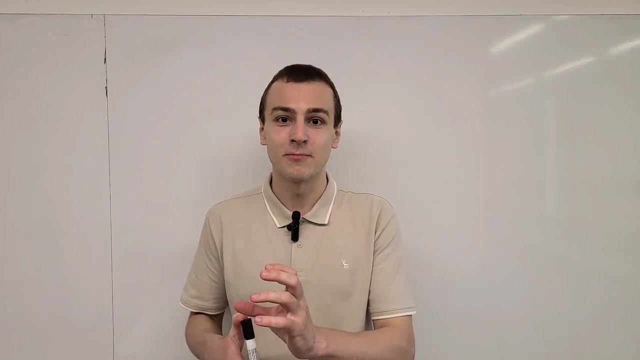 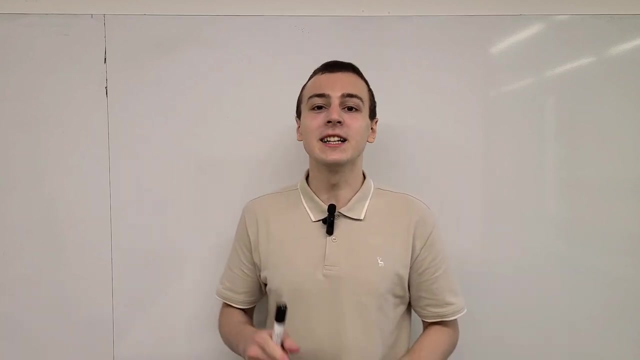 Let's see how the Hadamard gate allows us to move between the Pauli Z eigenbasis and the Pauli X eigenbasis. The Hadamard gate is an operator that acts on qubit states. These are states that are part of a two-dimensional Hilbert space. Let's begin by defining the Hadamard gate. 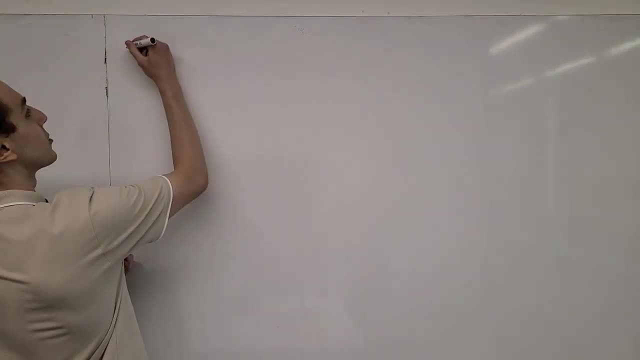 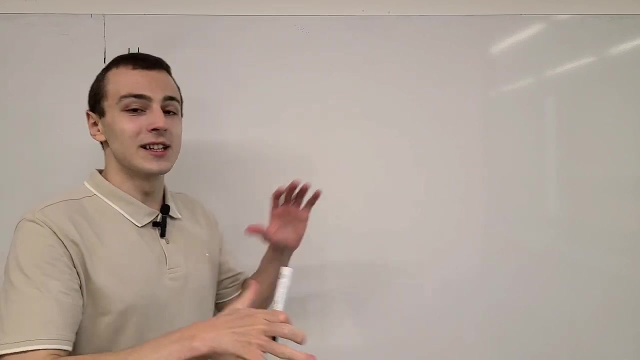 We can denote the Hadamard gate by capital H. Now there is some confusion here, because capital H is also used to denote the Hamiltonian in quantum mechanics and H is also used to denote Hilbert spaces. So the same letter is used to denote these very different concepts, But in this context over. 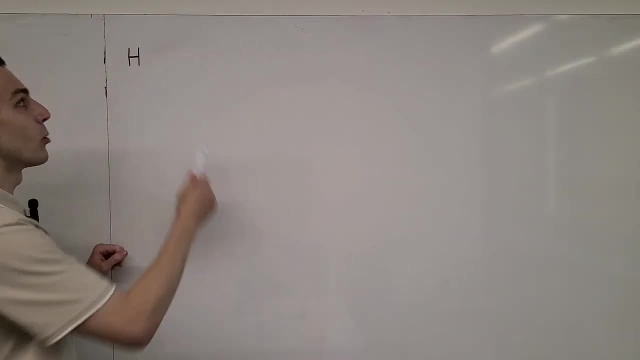 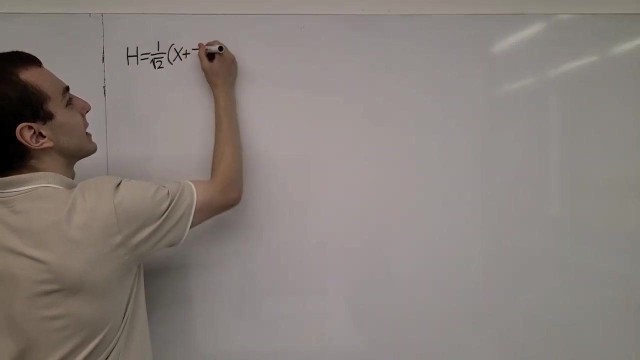 here we are denoting the Hadamard gate with the capital letter H, And we can define this in terms of Pauli matrices. This is 1 over the square root of 2 times the sum of Pauli X and Pauli Z. 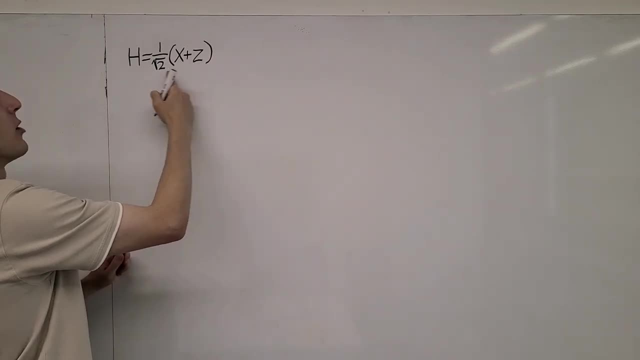 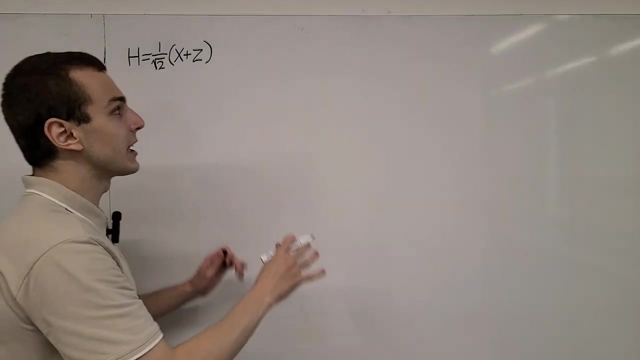 So these are the familiar Pauli matrices, And over here we have a normalization coefficient, And we'll see why this coefficient is needed in the definition, because it makes a lot of the equations and relationships later much more convenient. It gets rid of annoying factors. 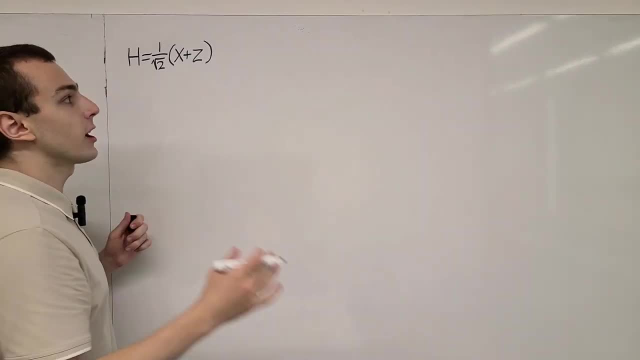 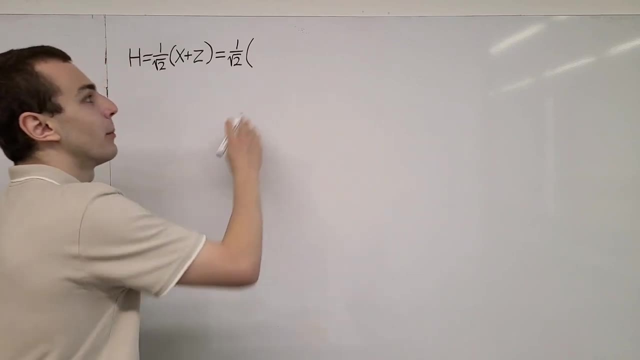 out the front. So let's look at the equations and relationships later. So let's look at the front. We can also write this in Dirac notation, And I'll do that over here. This is equal to the same normalization coefficient. And then we have a bunch of ket bra combinations. So first I'll 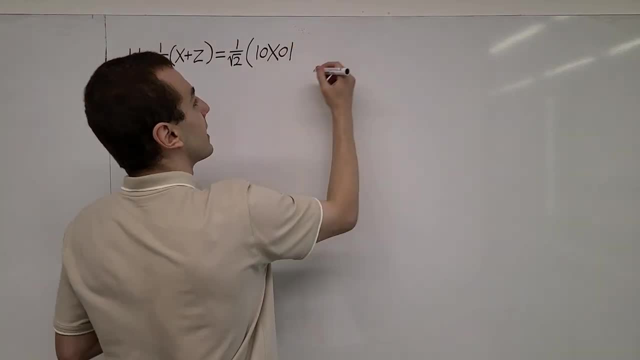 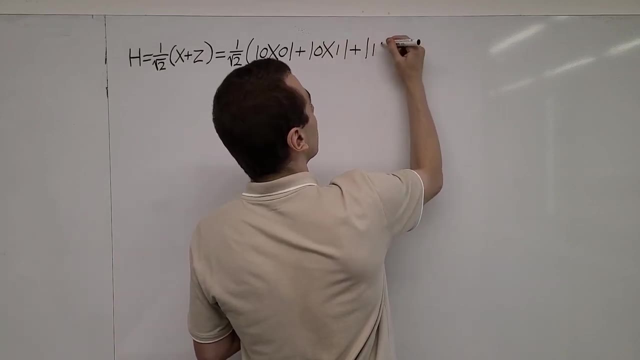 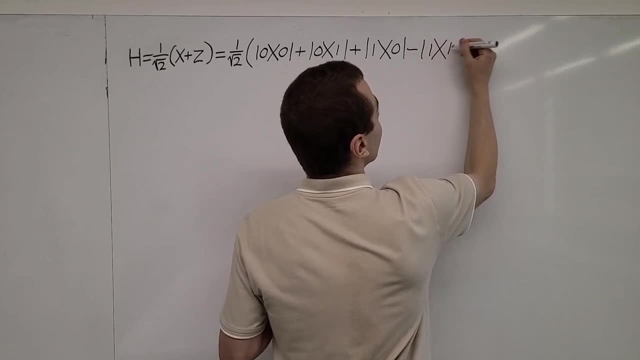 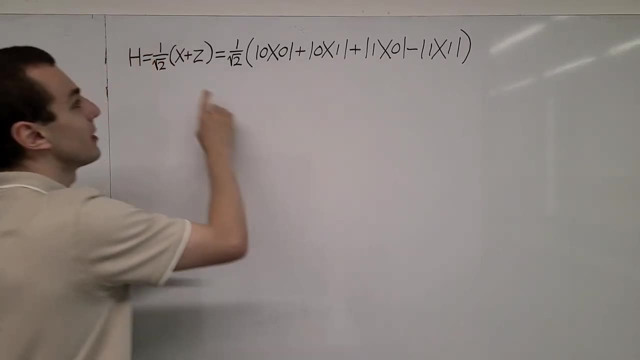 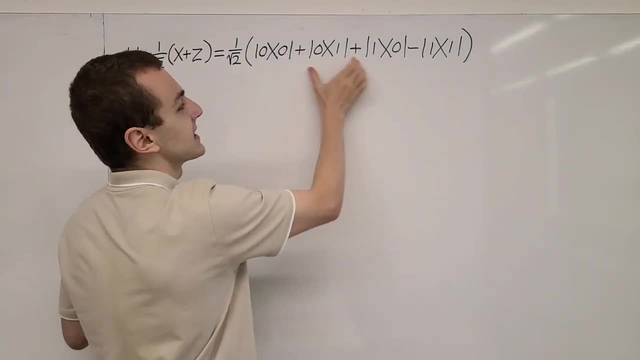 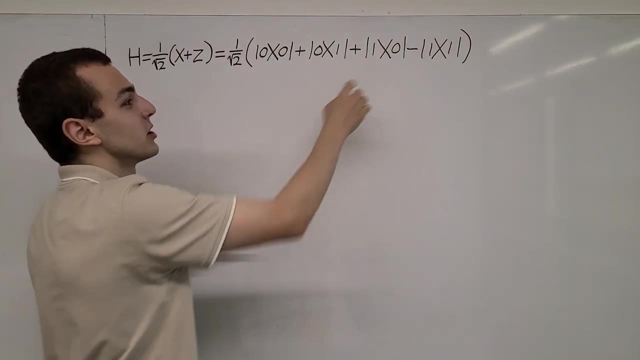 operator. So the Pauli X operator is defined as the sum of these middle two operators. If we were to put this in a matrix representation, these would correspond to the off-diagonal entries, So the non-leading diagonal entries. they would correspond to these two entries. 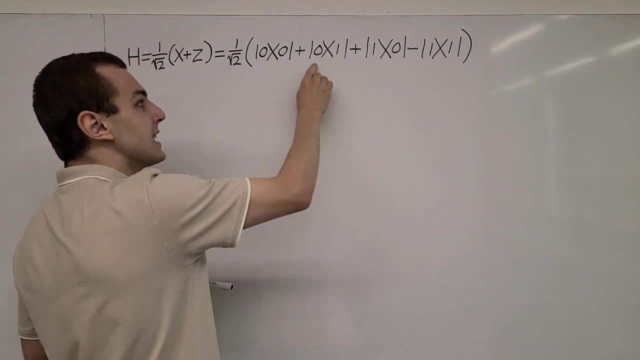 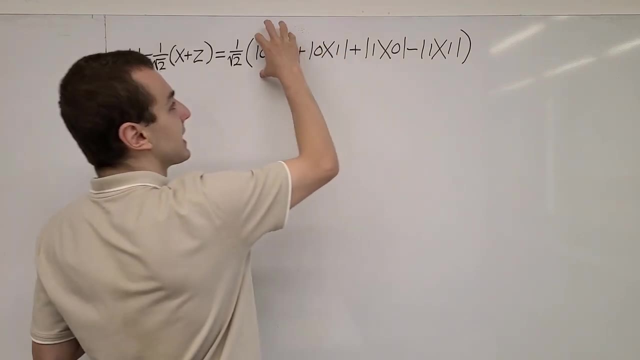 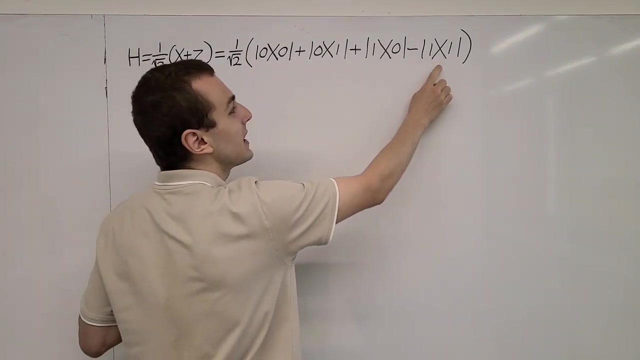 to these two values over here And when we have a ket-bra combination that gives us an operator. Now, what about this combination and this combination over here? Together, this combination and this combination, they are diagonal entries And we can see a plus one over here and a minus. 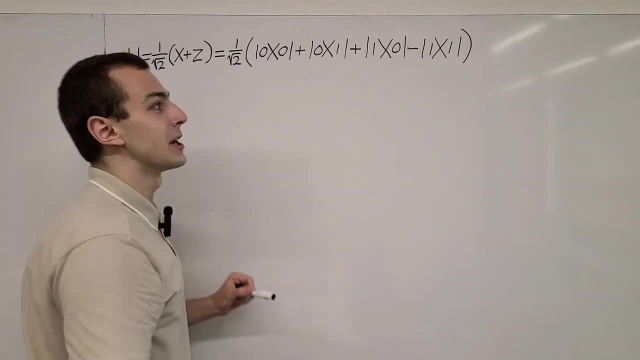 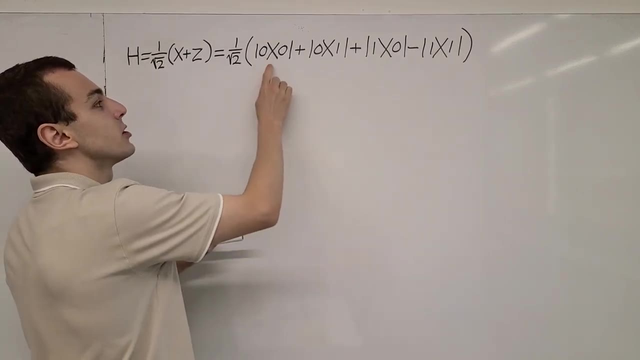 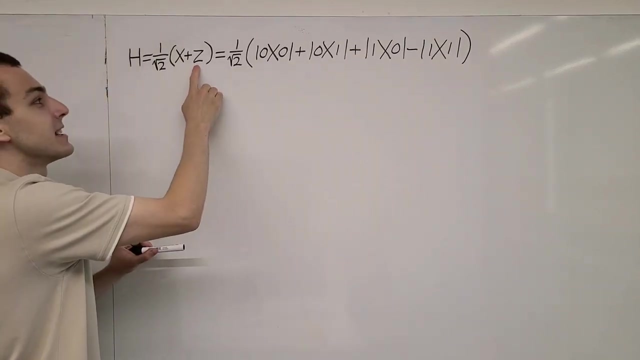 one implicitly, as the coefficients of these ket-bra combinations. So these are diagonal elements if we put this in a matrix representation, So this would correspond to a diagonal matrix that has entries one and minus one And that is the Pauli z, So those two ket-bra combinations. 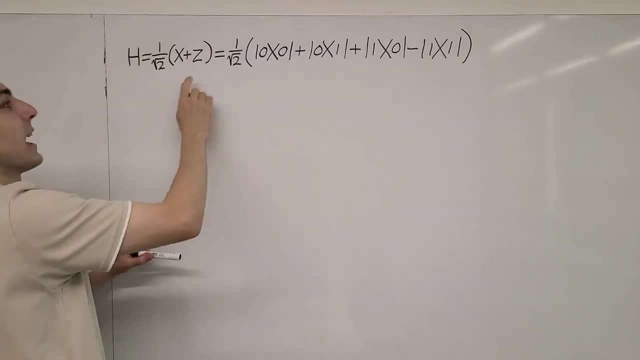 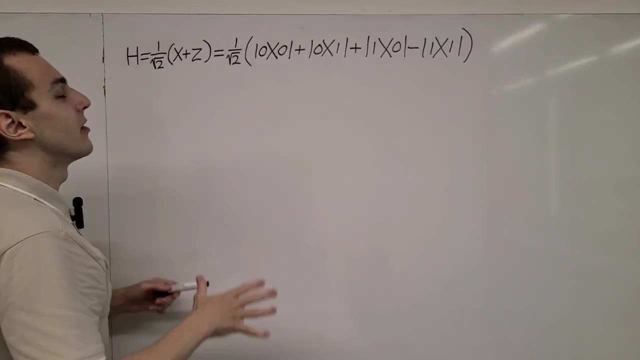 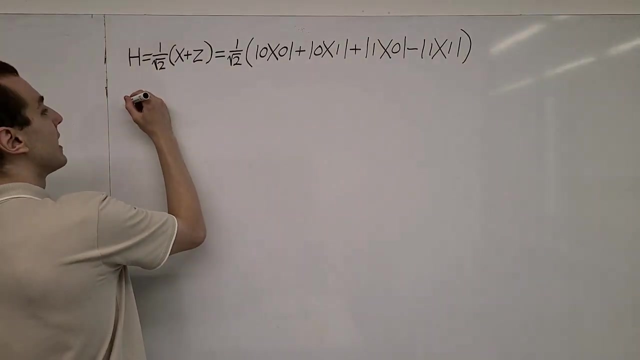 come from the Pauli z And if we take the sum and then divide by this normalization factor, then we get the Hadamard gate. Now let's see the matrix representation and how it acts on a general qubit state. So we're going to take the Hadamard gate and we're going to act on a ket. 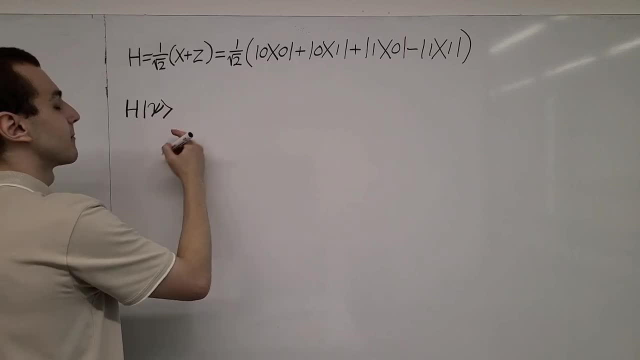 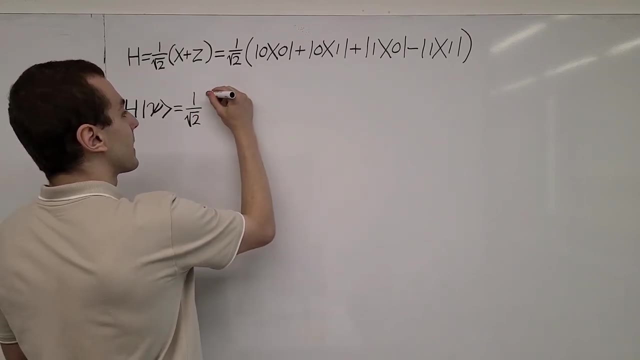 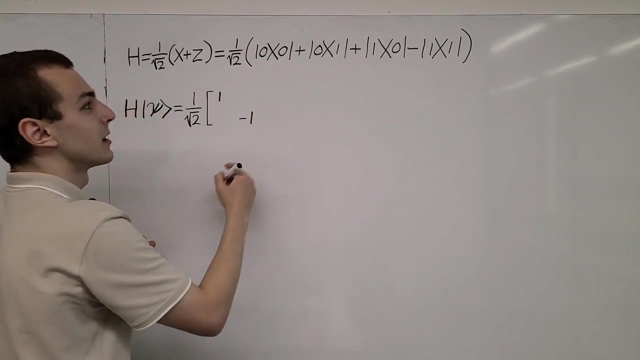 So this is some general qubit state And in matrix representation we're going to have one over square root of two. That's the same normalization factor. And then we're going to have the matrix, And the matrix has diagonal entries one and minus one. That's this and this. 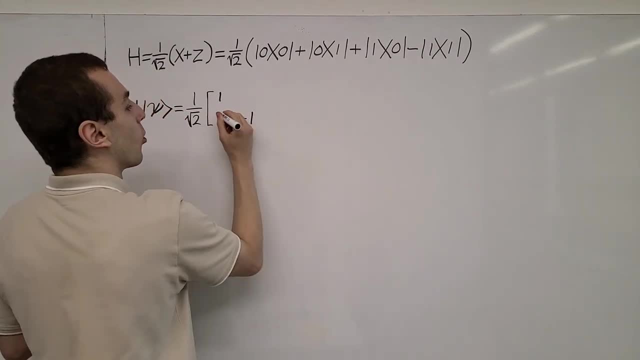 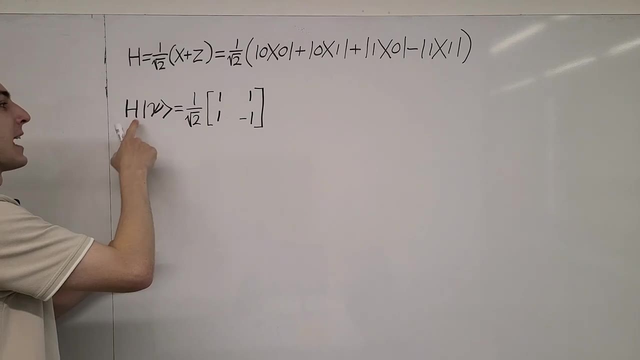 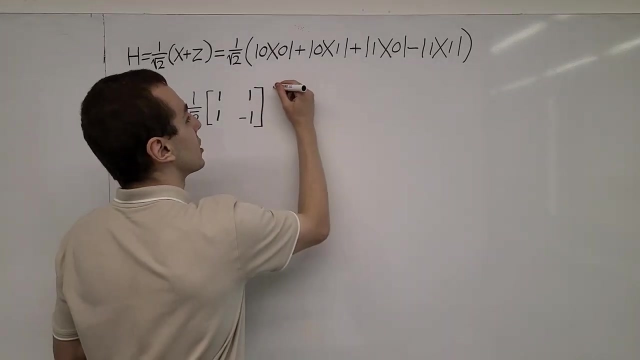 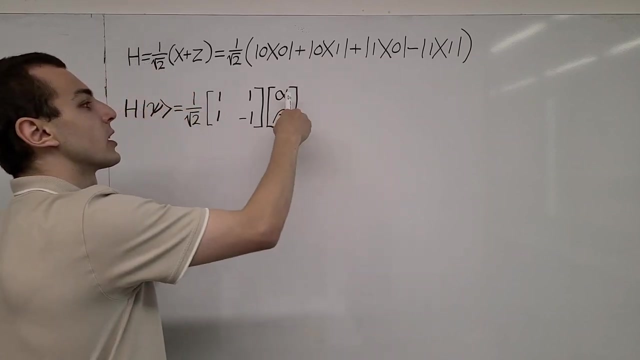 over here And off diagonal entries. they are also one and one. So this is the matrix that represents this operator And this Hadamard gate has this specific matrix representation. And let's act on a general state And we'll use the coefficients alpha and beta to denote the coefficients of the computational. 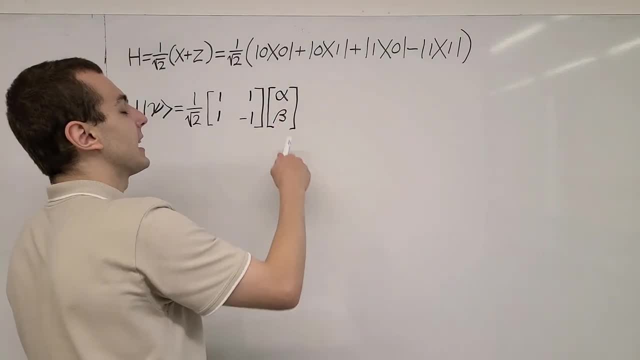 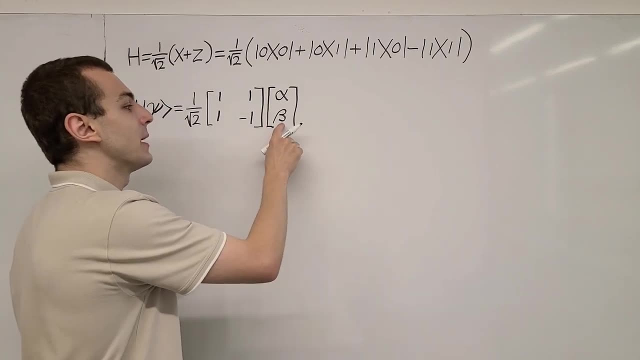 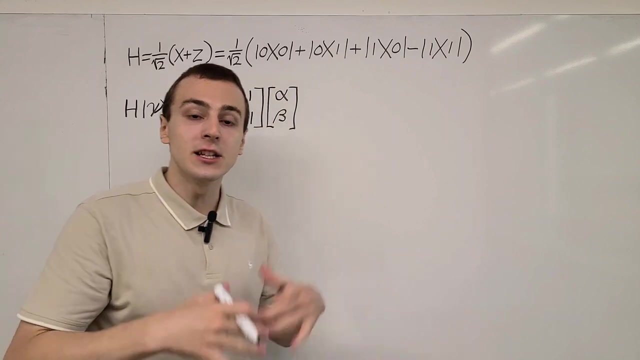 basis states. So this alpha is the coefficient that multiplies the zero ket, So it's the ket labeled by zero, And beta multiplies the ket labeled by one, And together they form the computational basis. We only need two computational basis vectors because this is a two-dimensional. 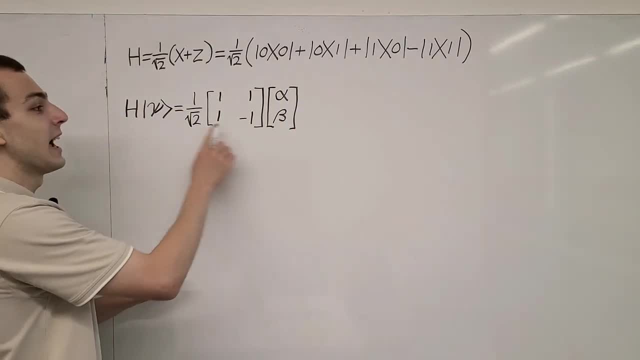 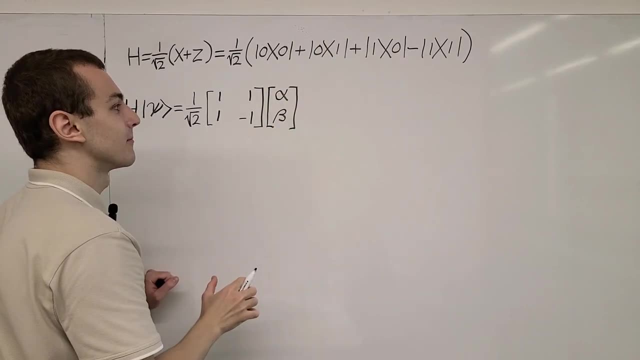 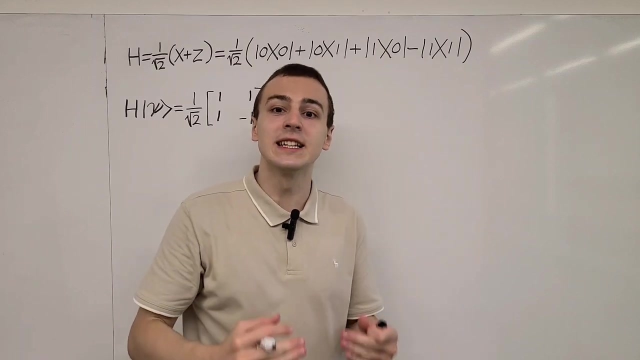 Hilbert space. The Hadamard gate over here acts on a two-dimensional Hilbert space And specifically it's acting on a qubit state. So alpha and beta also have to satisfy the normalization condition, And we impose the normalization condition to get rid of any of those annoying factors that would 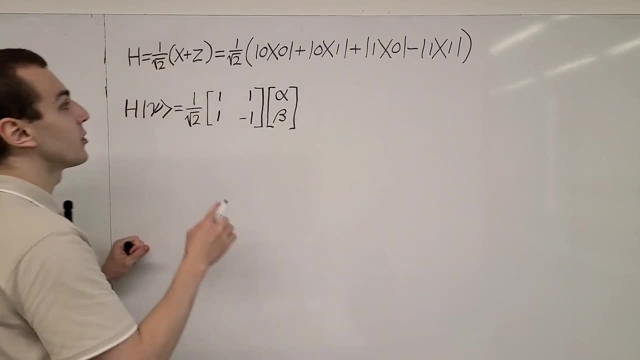 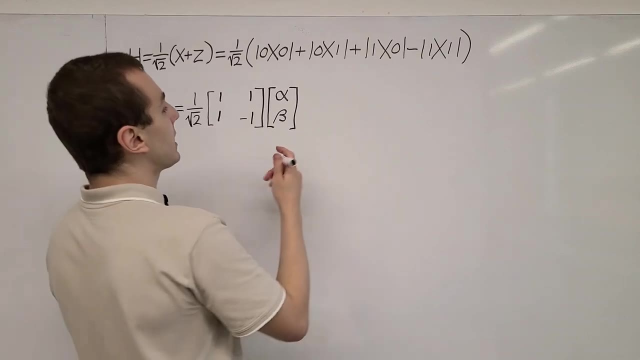 appear at the front And we have to satisfy the normalization condition And we impose the front of relationships. That's also the reason we have this coefficient at the front over here. It is to preserve normalization. So let's see what we get when we actually perform this matrix. 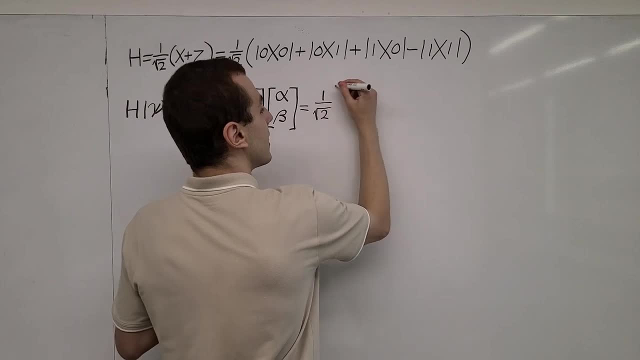 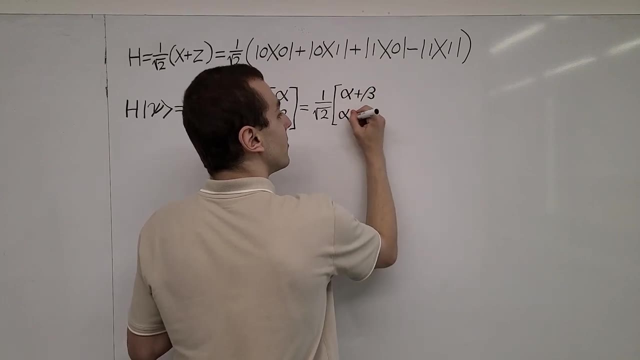 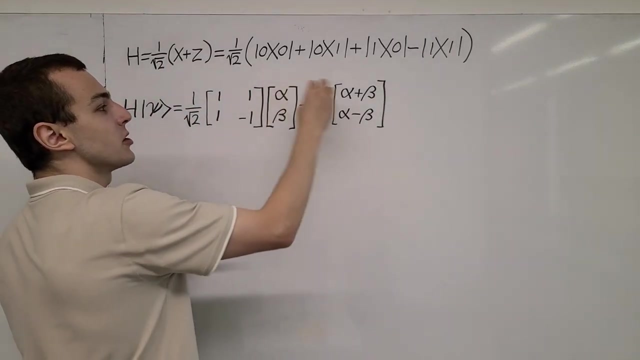 multiplication. We're still going to have this factor out the front, but on the inside we're going to get alpha plus beta and then we're going to get alpha minus beta. Those are the two entries. So you can see that this alpha has now turned into a sum and this beta has now turned into a. 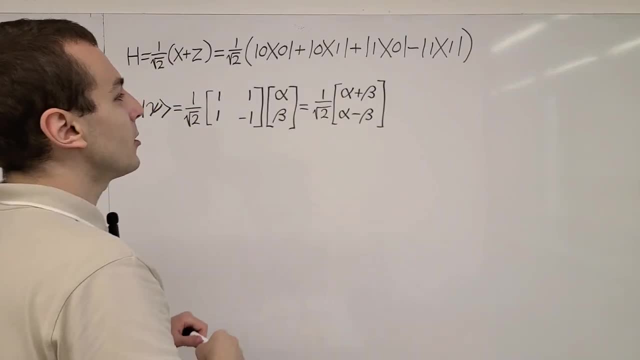 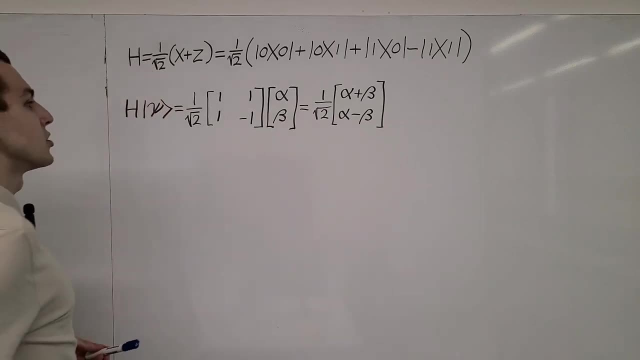 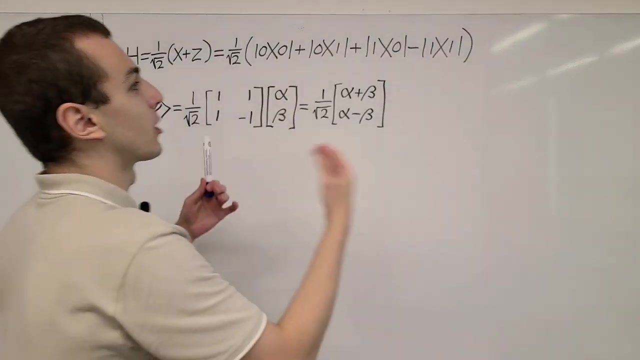 difference of the coefficients. And there is another way we can actually write this. We can write this in an alternative way and I'll write that underneath over here. So what is this actually telling us? It's telling us that if we take this state over here, which is the ground state or the 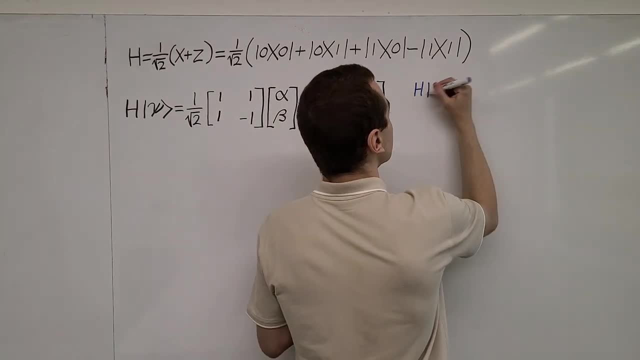 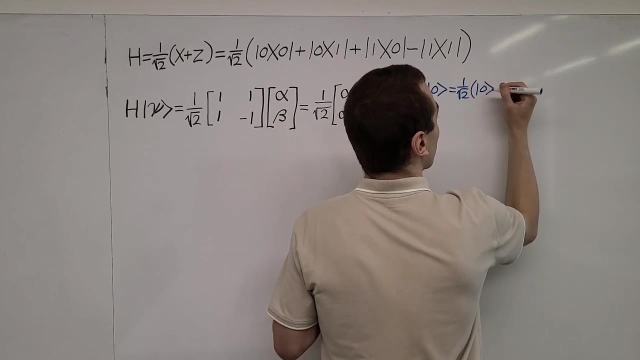 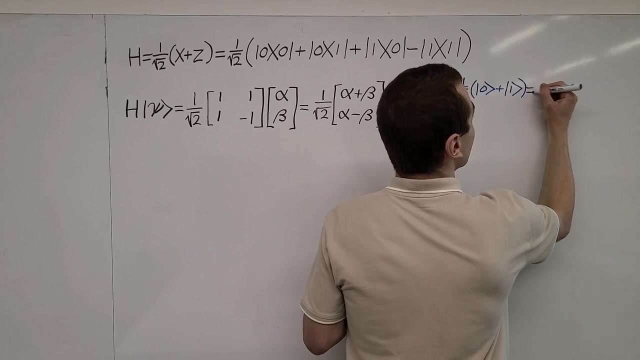 state labeled by zero and we act with the Hadamard gate. that's going to give us the plus one on the square root of two times the sum of this computational basis state and the computational basis state labeled by one, And this is the same as plus the ket labeled as plus. So 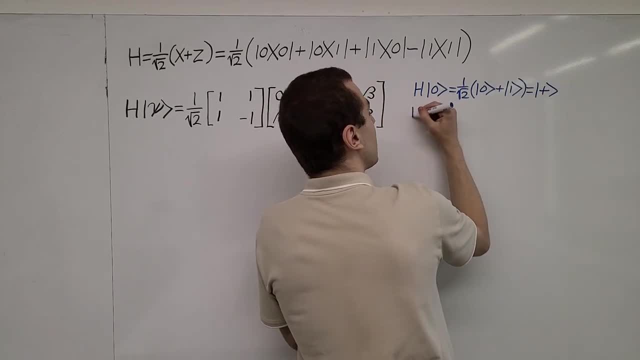 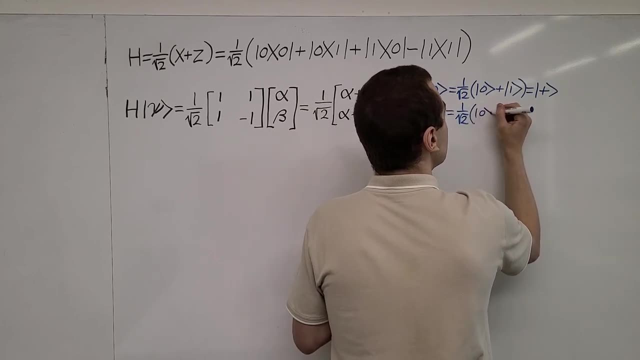 this is shorthand notation for this combination And for the other computational basis state, which is labeled by one. we have this combination, which is the difference rather than the sum. So we have a minus one over here and we have a minus one over here And we have a minus one over. 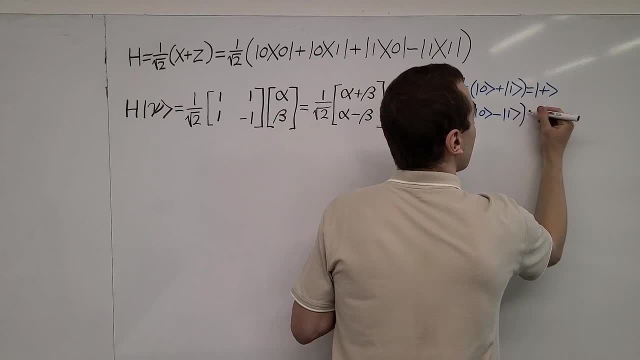 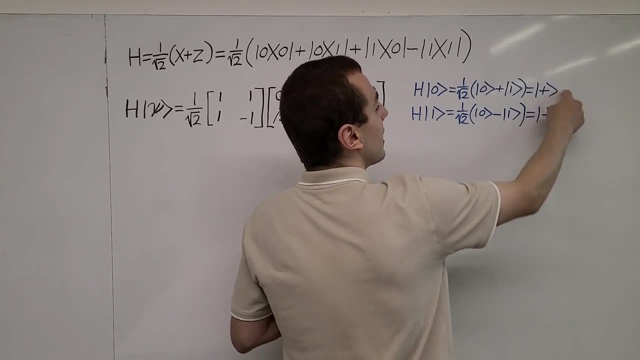 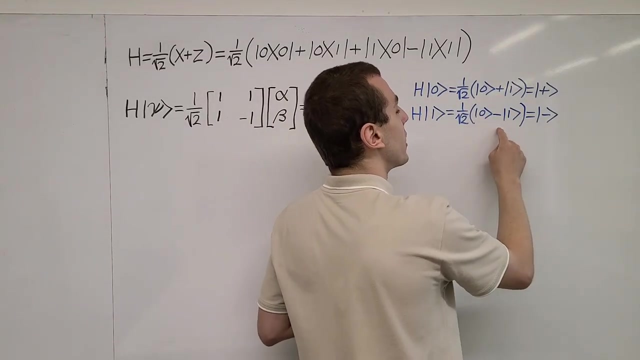 here and we have a minus sign on the state labeled by one, And we can call this minus over here. These two states are the eigenstates of the Pauli x operator. They have eigenvalue plus one and minus one respectively. So if you took this Pauli x operator and you acted on these states, 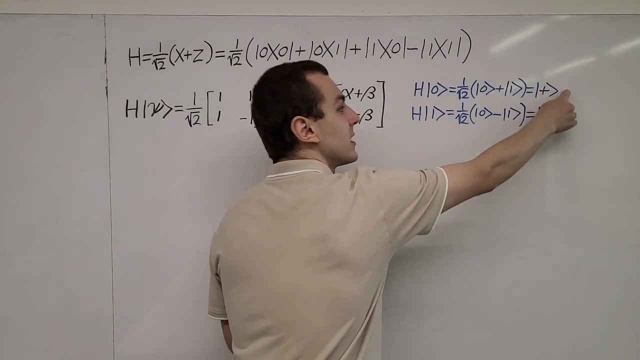 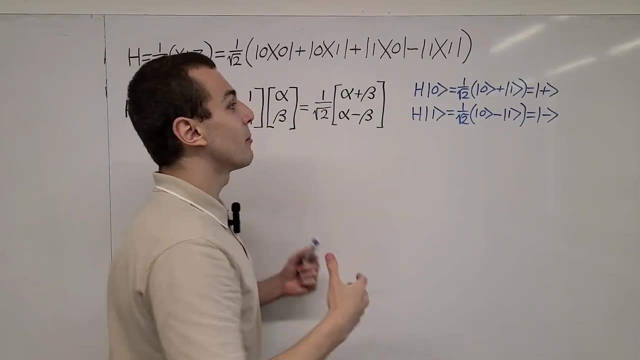 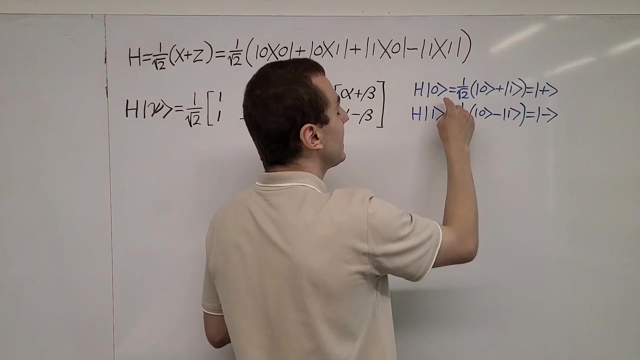 you would get back the same state with an eigenvalue of plus or minus one, And these computational basis states, they are the eigenbasis of the Pauli z operator. So that's this Pauli z operator. So the Hadamard gate has changed these Pauli z eigenstates to Pauli x. 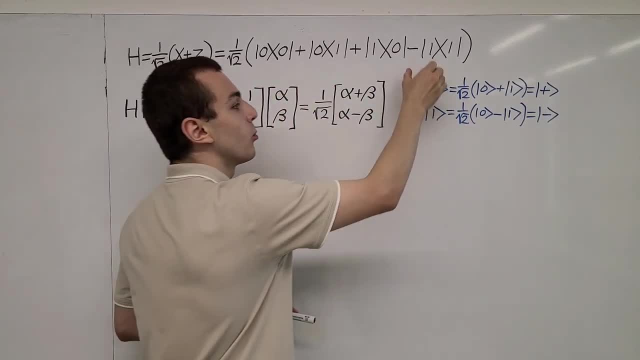 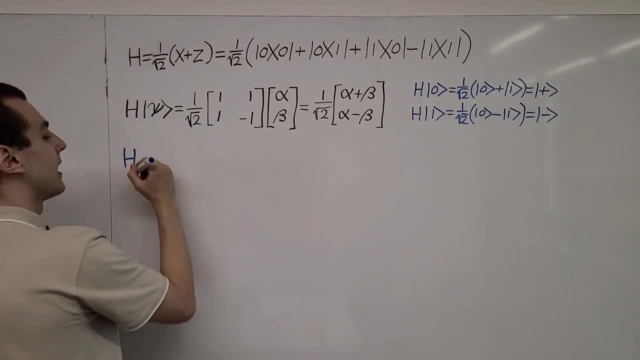 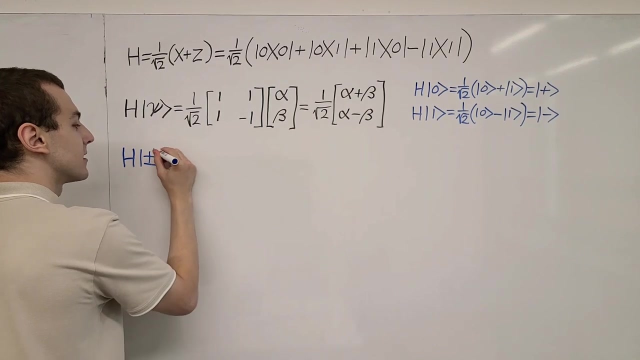 eigenstates. Let's see what it does when we act on these two states. So I'll write that down over here. If we take this Hadamard gate and we act on either the plus or the minus for a general, I'll write this out generally. So we'll have plus and minus inside here. So we take 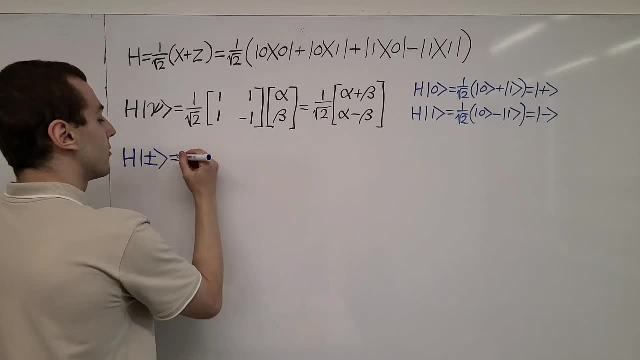 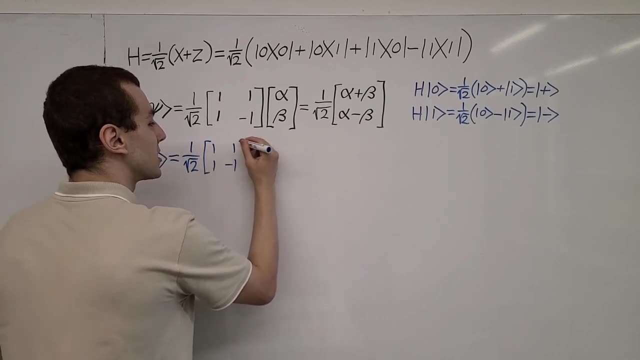 this ket and we act on it. What is that going to give us? Well, if we write this out in matrix form, we're going to have this same matrix. So one one, one minus one, And it's going to act. 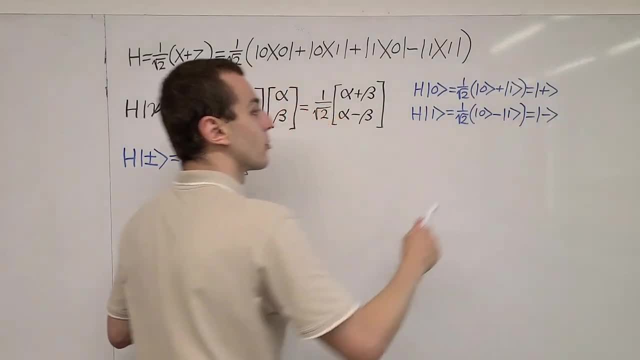 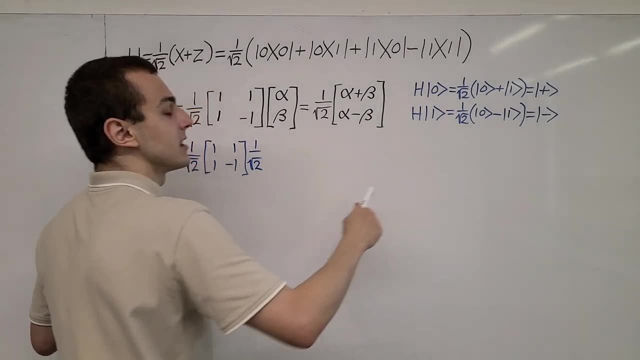 on these two states And let's let's write these states in their matrix representations. So we're going to have another factor of square root, one on square root of two, that comes from there, And then we're going to write this out in matrix form. So we're going to have this same. 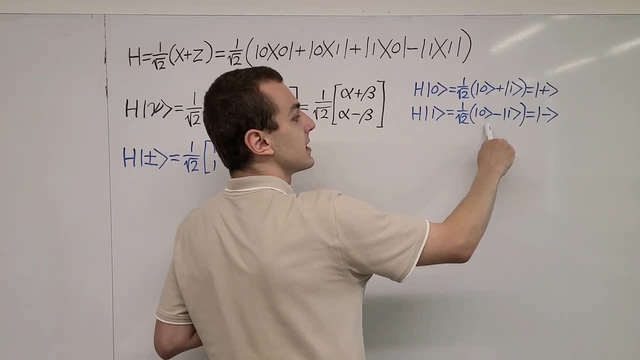 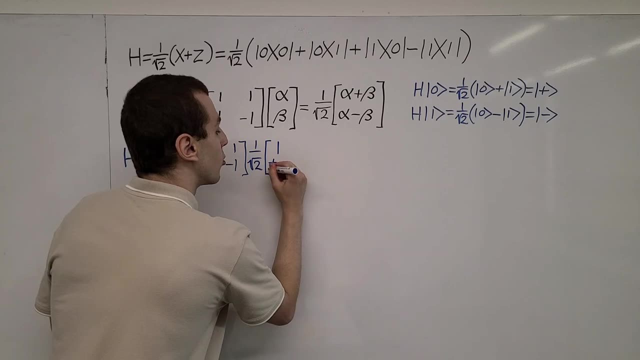 matrix representation. So we're going to have this same matrix representation. So we're going to have one as our first entry that represents this zero state, the state labeled by zero, And then the next state is going to be plus or minus one, And this sign depends on whether we're dealing 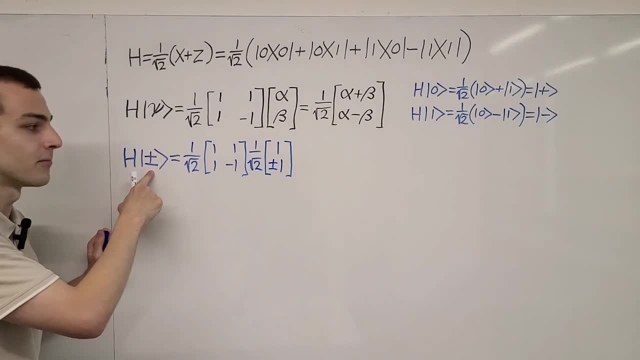 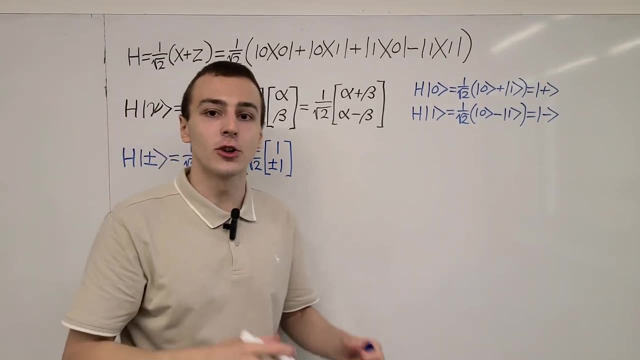 with the plus or the minus version of this ket. So all of these labels in the kets, they are just labels. we could put any symbol in there as long as we're consistent. So this zero and this one, they're just labels. 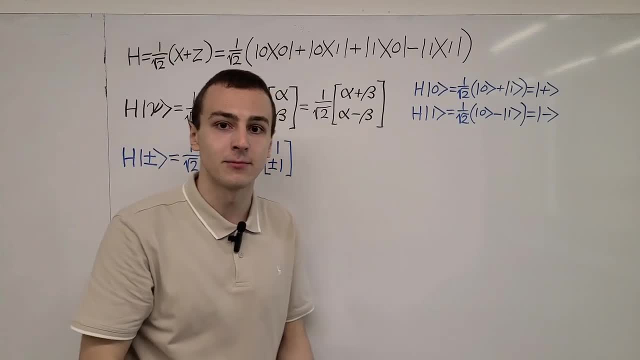 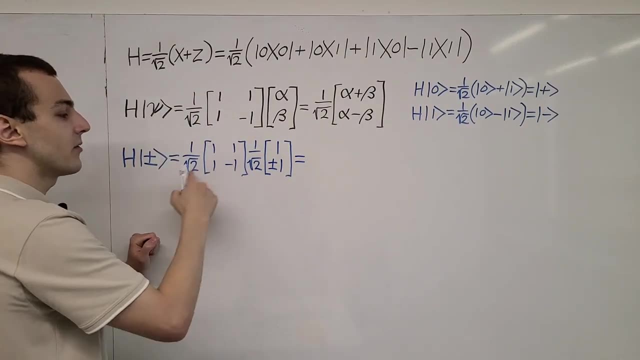 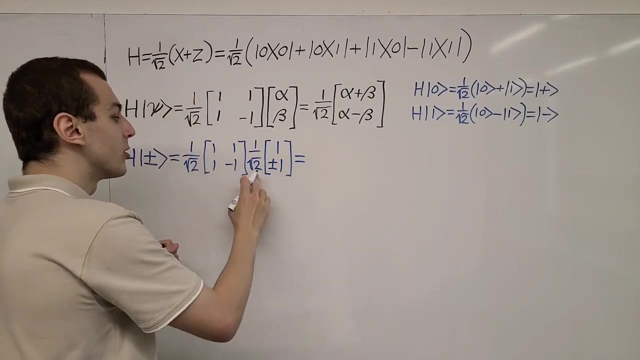 For the two possible states in the computational basis. So this is what we get. And if we multiply this out, what are we going to get? Well, this factor and this factor can be combined together. we're free to move constants around because they satisfy commutativity. they are real numbers. 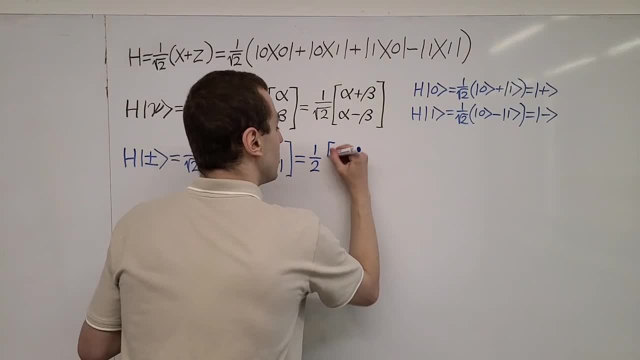 And so that's going to give us one half, And over here what we're going to get is one times one plus one times plus or minus one, So we're going to have one plus minus one, But when we perform this other multiplication we have this minus sign here. 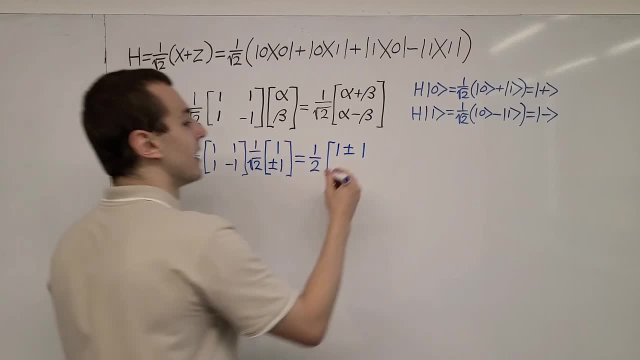 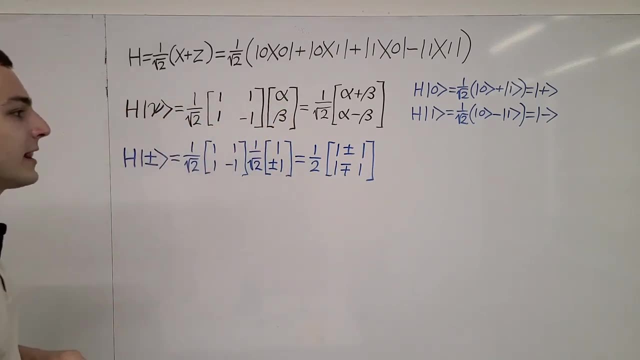 And this minus sign is going to flip this plus minus sign and it's going to turn it into a minus plus sign. So this is what we're going to get, And we can write this out slightly differently. So this is a general equation that works for both plus and minus, But if we separate this, 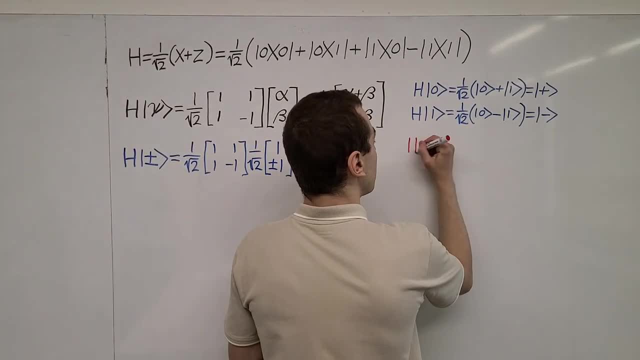 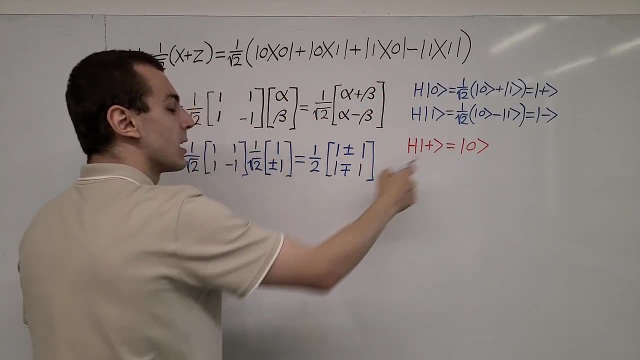 out into the two cases. what happens is, if we act with h on this plus state, we're going to get the zero state. Now, where is that coming from? Well, if you look at this case, if we just focus on plus and we treat- treat this over here- as a plus, 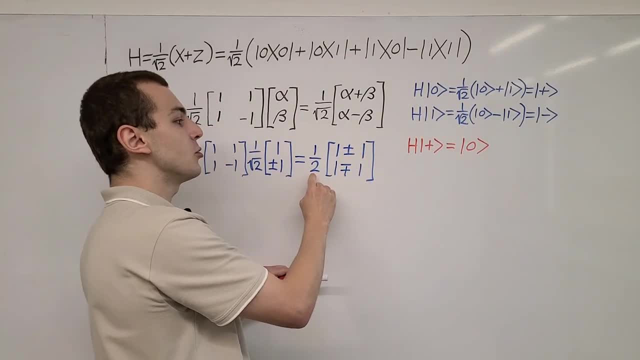 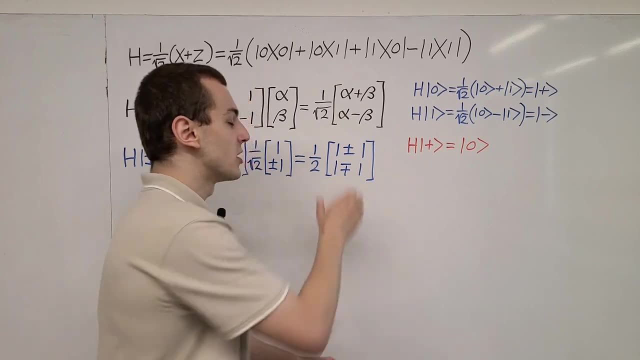 that's going to give us one plus one, which is two. we divide that by two, that gives us one, And over here we're going to use this minus and we're going to have one minus one, which is zero. So then the matrix that we get is a column vector that has entries one zero And the. 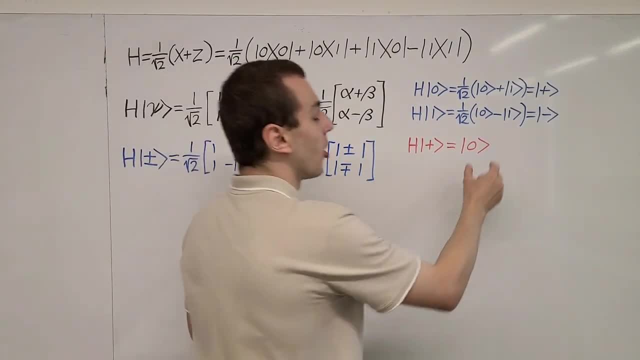 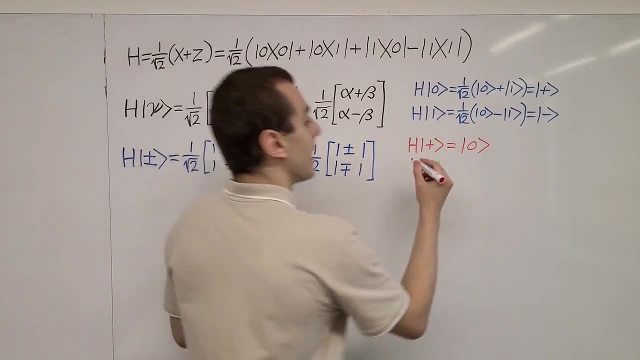 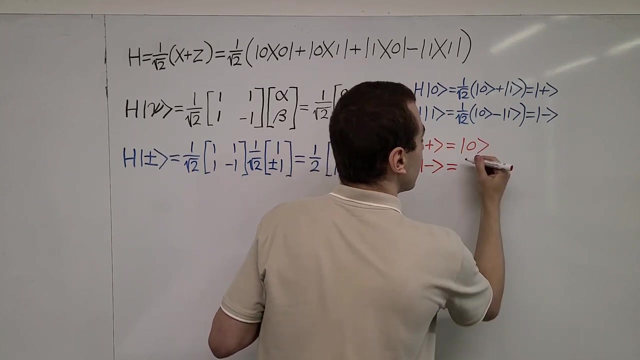 one zero, that column vector, that is the matrix representation of this ket in the Pali z eigenbasis. So that's what we're dealing with here, And if we act with the Hadamard on the minus case, so in this minus ket, then what we're going to get is one. we're going to get the ket. 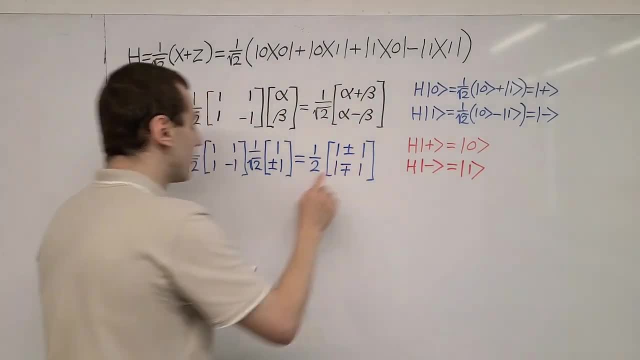 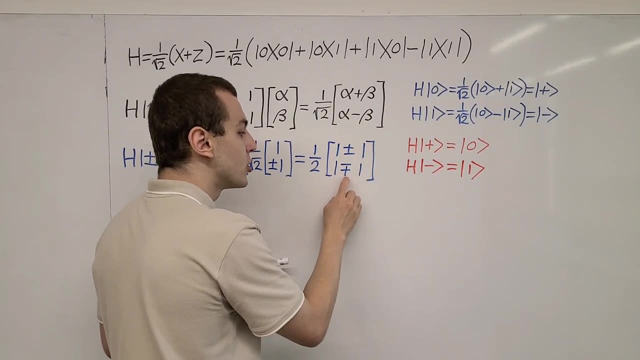 labeled by one, And we'll go through that case. If, instead, we had a minus over here, then we would choose this minus. we'd have one minus one. that would be zero in the top. And if we here, we would choose the plus, that would give us one plus one. that's two divided by two, and we 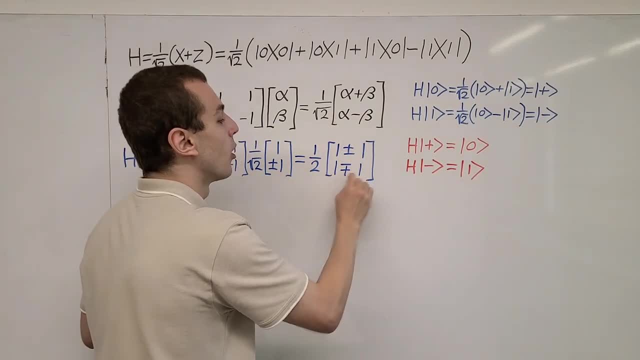 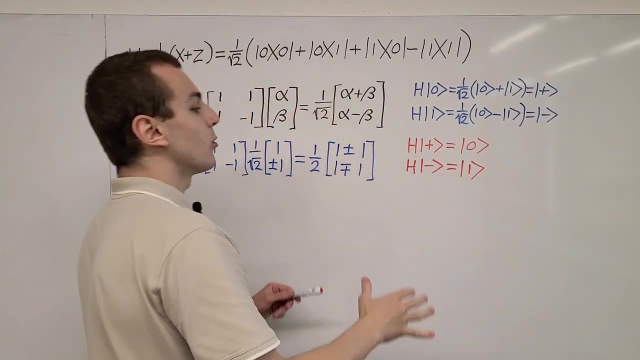 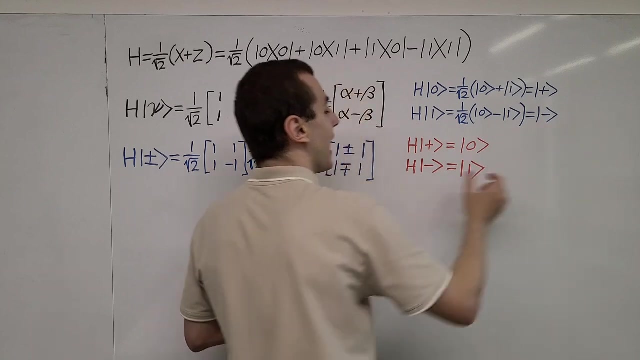 have one. So then we would have the entries zero one in this column vector And that is the matrix representation of this ket. So you can see that we are moving from the Pali z eigenbasis to the Pali x eigenbasis And over here we're moving from the Pali x eigenbasis to the Pali z eigenbasis. 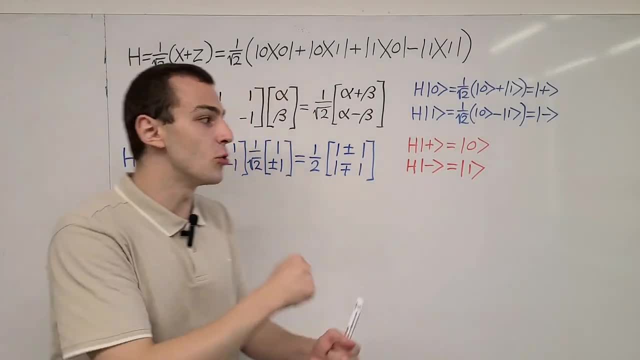 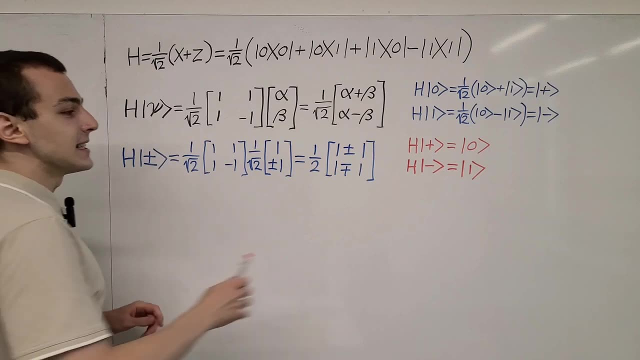 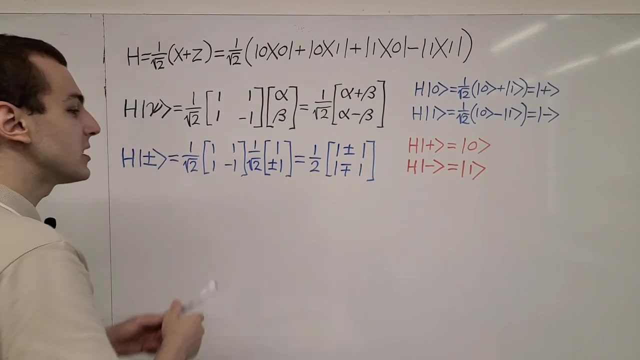 The Hadamard gate allows us to shift between the Pali z eigenbasis and the Pali z eigenbasis, So now what I want to do is examine another way of writing this. Instead of writing it in this form, we could actually sandwich the operator in between two Hadamards, Because the Hadamard gate 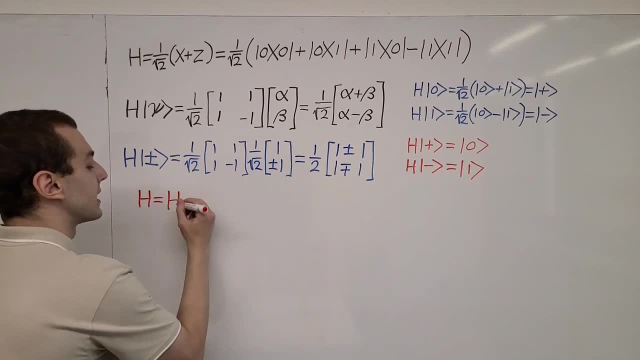 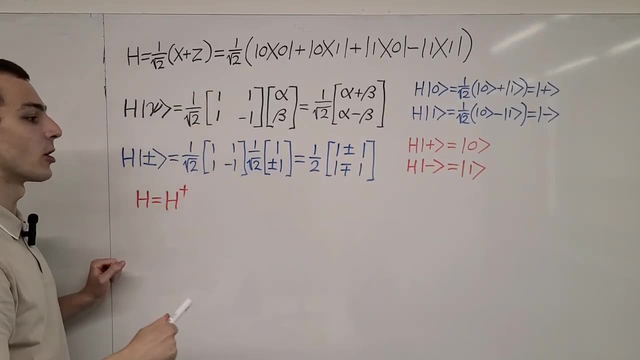 is Hermitian. the Hadamard gate satisfies this property. it is Hermitian, So let's go ahead and sandwich Pali x and Pali z between Hadamards. So if we do that, then what we're going to get is: 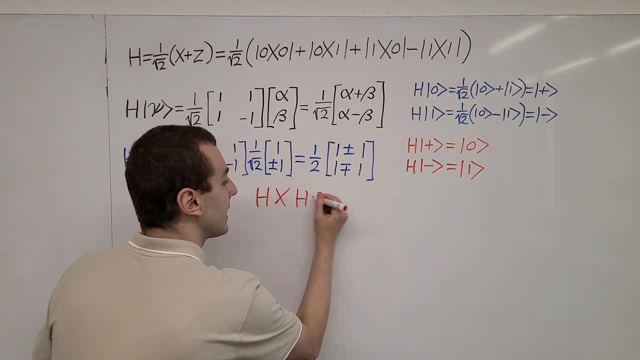 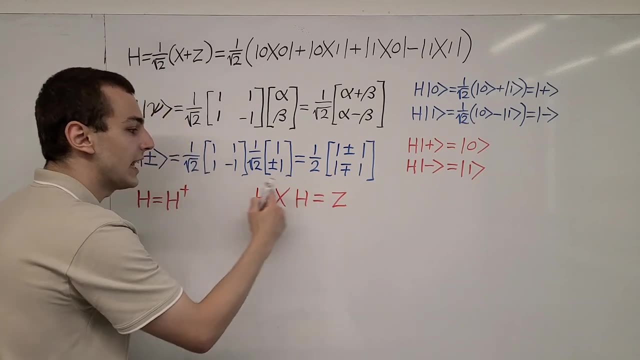 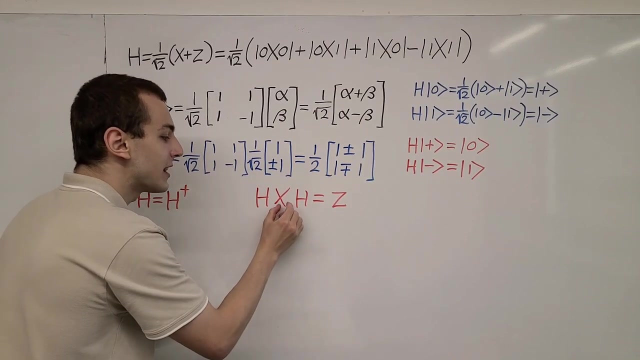 h, x, h equals z. Now this h and this h are exactly the same. we could put a Hermitian adjoint on either one of these and that would give us the exact same result. So this is how you would transform this operator. We're transforming this operator with this unitary transformation. We're 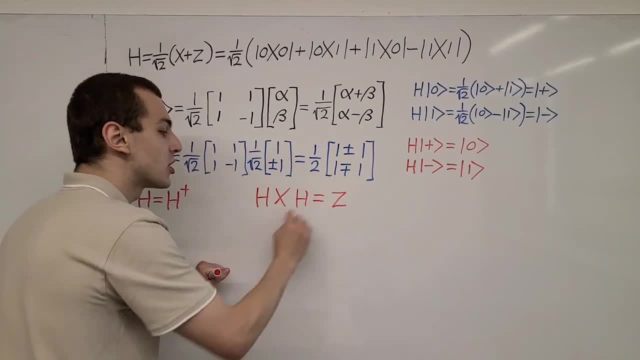 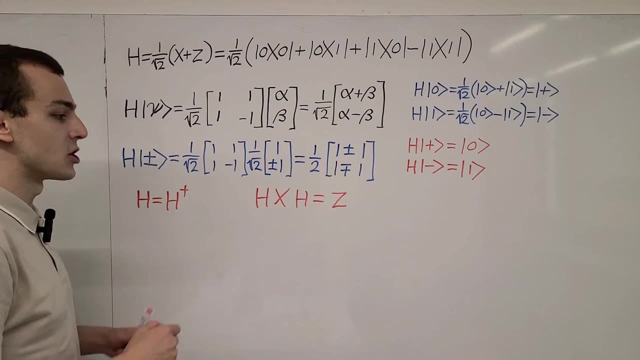 treating the Hadamard gate as a unitary transformation that allows us to go from Pali x to Pali z. Now what I want to do is write a slightly different way of writing this. So let's write a slightly different form of this equation. I'm going to act on both sides, from the left and 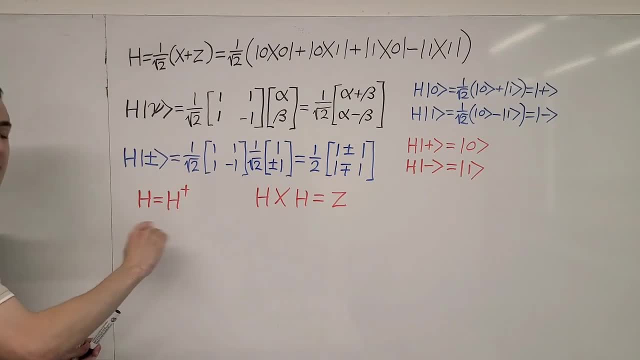 from the right, with the inverse, which is the same. It's the same as the Hadamard gate. And if I do that, I'll show you what I get. If I get, if I take h, dagger h, and then I put x in the middle, and then 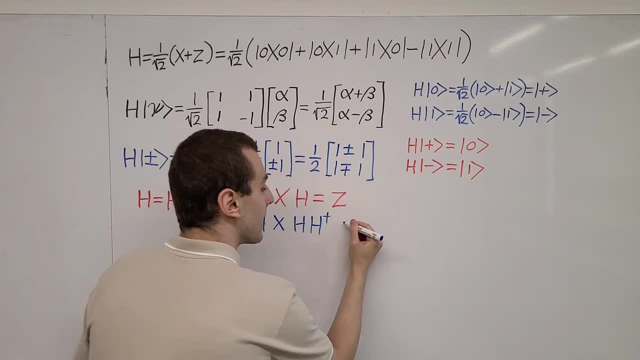 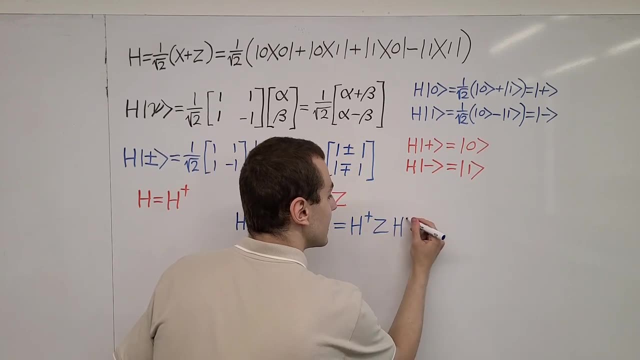 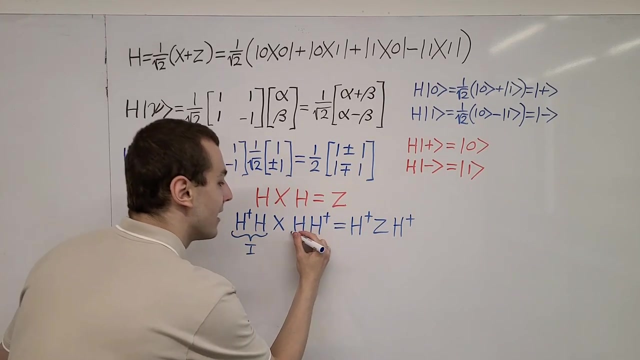 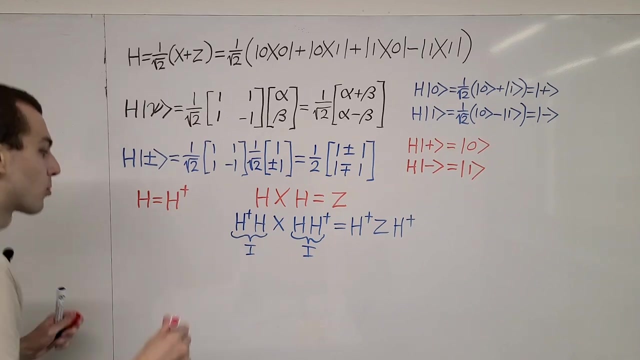 I put h over here and then follow that with h dagger. the right hand side is going to turn into h dagger And this combination over here is the same as the identity. And this combination is also the same as the identity. That's because the Hadamard gate satisfies another very useful 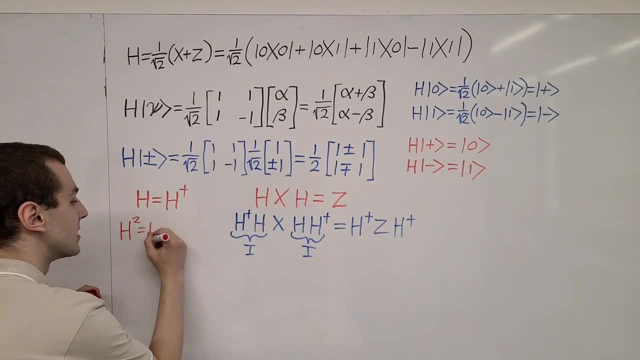 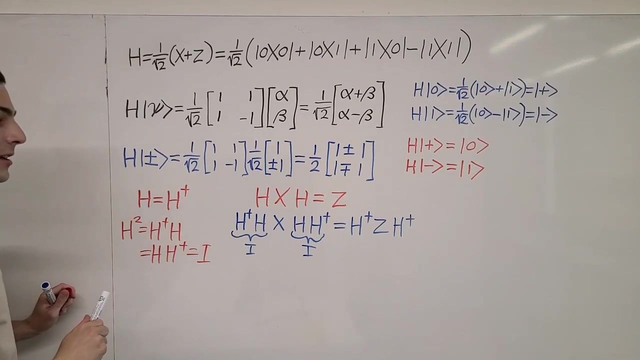 property where h squared, which is h dagger, h, that's also equal to h h dagger. this is equal to the identity. So the Hadamard gate also satisfies this property and it is also Hermitian. So now what we can do is we can also identify that this. 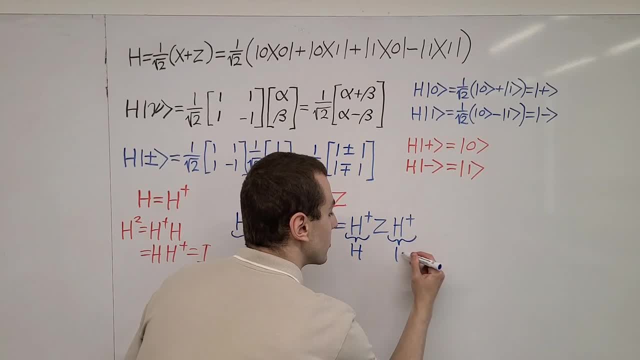 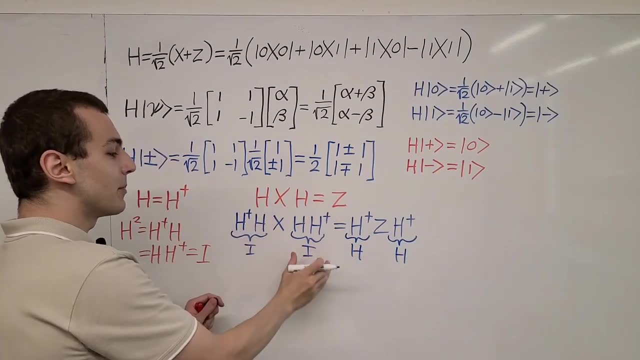 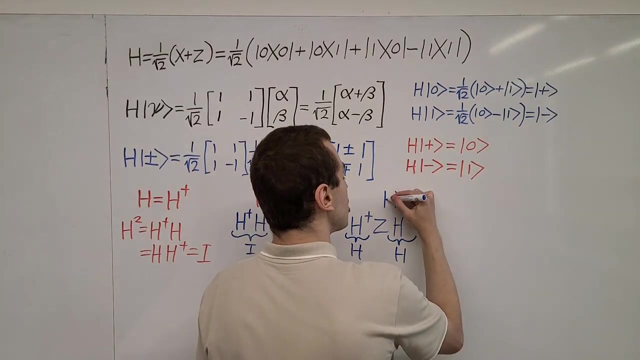 is equal to the Hadamard gate and this is equal to the Hadamard gate. So then, finally, what we see is that we get an analogous relationship where these guys disappear because it's just the identity, and then we sandwich z. So that gives us this relationship where we have h, z, h equals x. 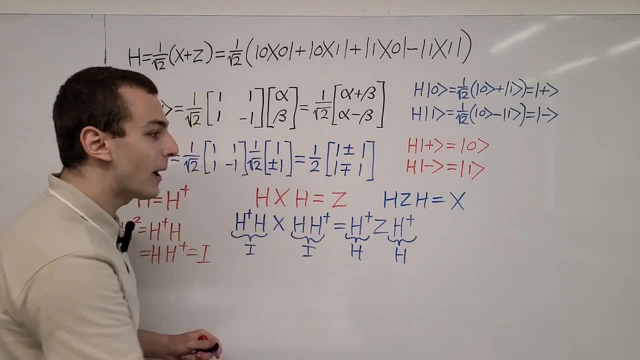 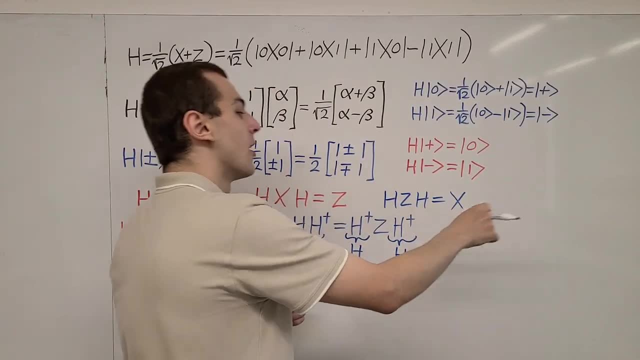 So it's an analogous relationship. If you sandwich either Pali x or Pali z in between two Hadamards, they will swap places. So the z will turn to an x or the x will turn to a z. Now, this property over here is also very. 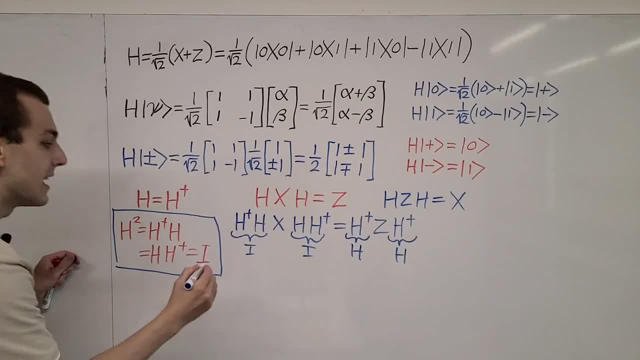 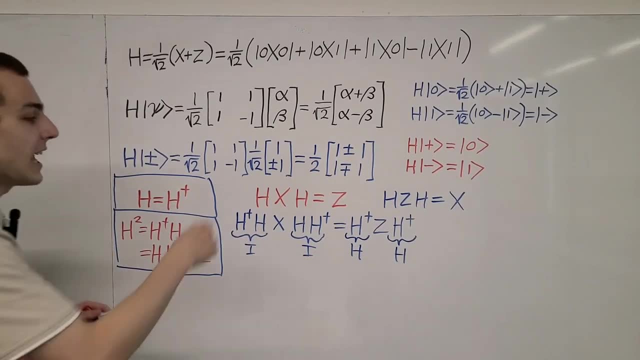 useful and we will prove this property in the next video in the quantum mechanics playlist. This property over here, the fact that the Hadamard gate is Hermitian, is immediately evident if you look at the matrix representation, If you perform the Hermitian relationship, you can see that the 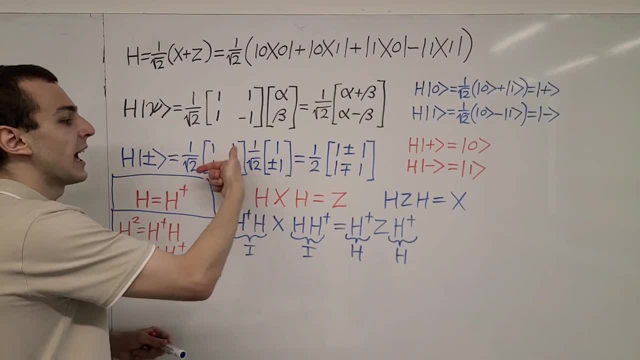 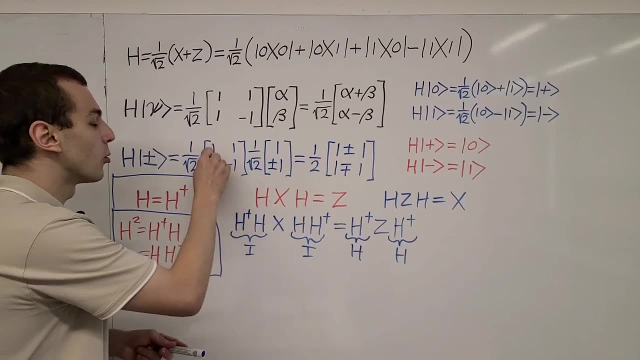 Hermitian adjoint. on this, you'll see that taking the transpose has no effect because this is a symmetric matrix, and taking the complex conjugate also has no effect, because all entries in this matrix are real numbers And the Hermitian conjugate of a real number is just itself. 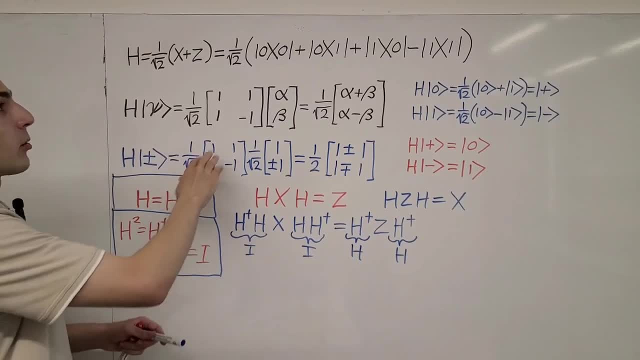 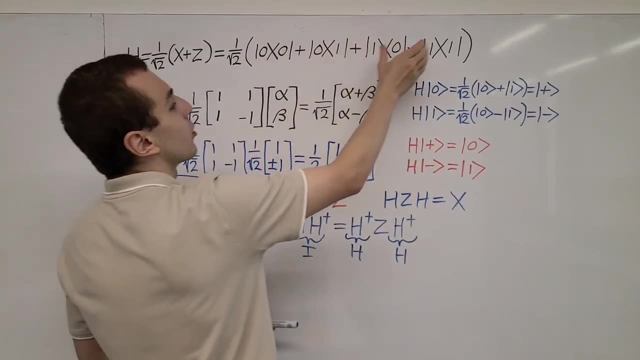 So over here we can immediately see that it is Hermitian. We can also see that it's Hermitian if we examine all of these guys over here. If we were to take the Hermitian adjoint of all of the Ketbra combinations, we would get back to the Hermitian relationship. So we can see that the 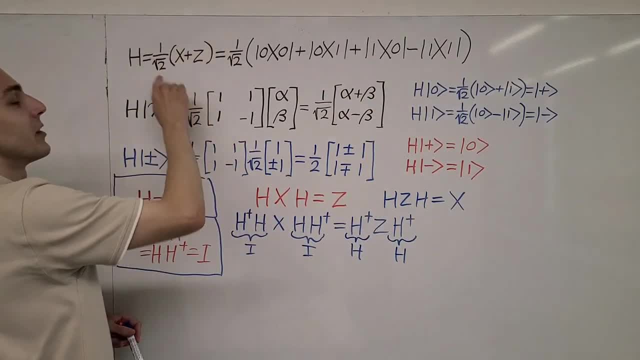 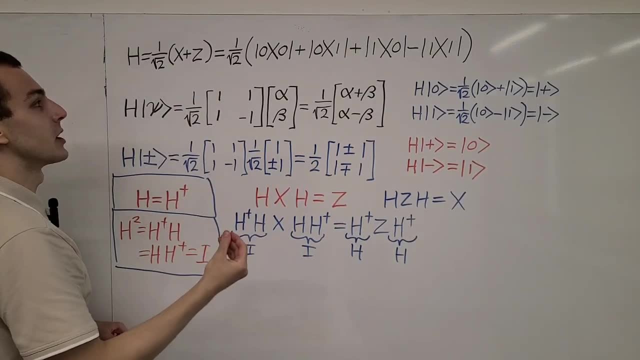 Hermitian relationship is exactly the same combination And if we look at this definition over here, we know that Pauli x and Pauli z are both Hermitian. The Pauli matrices are all Hermitian. So if we take the Hermitian adjoint of these two matrices, we're going to get back exactly the same. 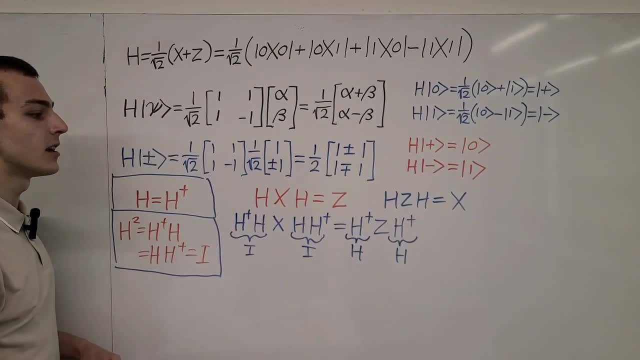 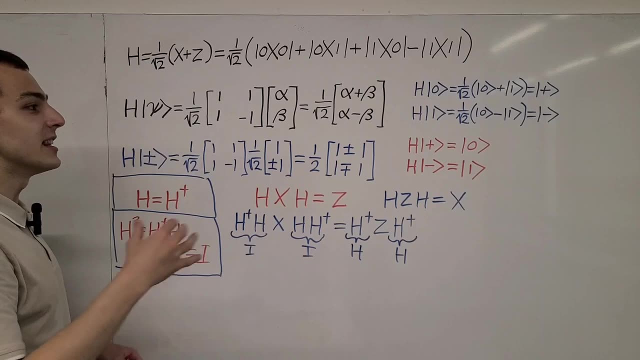 thing. So in the next video in the quantum mechanics playlist we're going to keep looking at the Hadamard gate and we're going to see some other interesting properties that the Hadamard gate has. In this video we've examined the Pauli x. 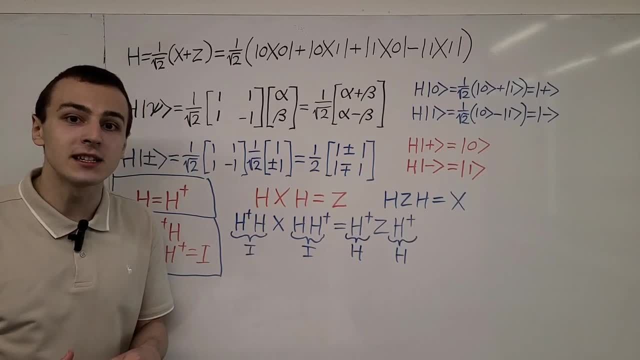 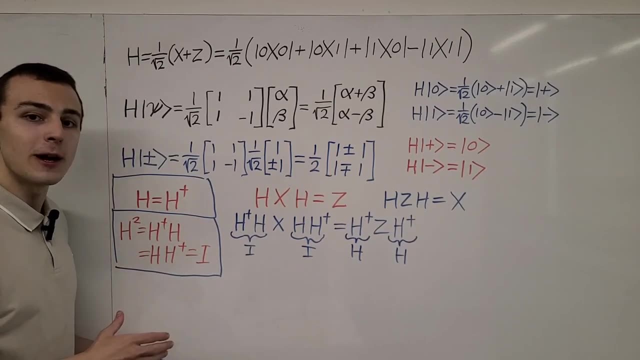 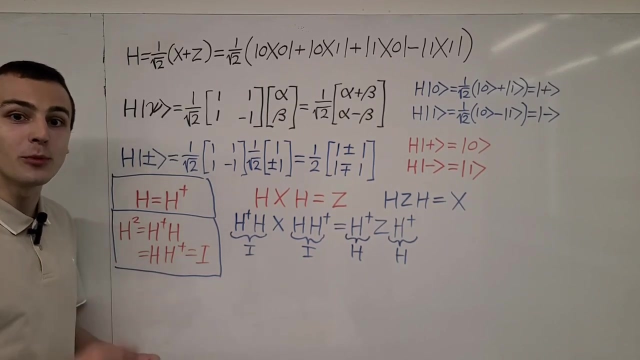 and Pauli z eigen bases, And we've seen how the Hadamard gate allows us to translate between these two useful bases. And this is essential mathematics for describing a two-dimensional Hilbert space. And that is the system that describes a qubit, a single qubit by itself. You can find all the